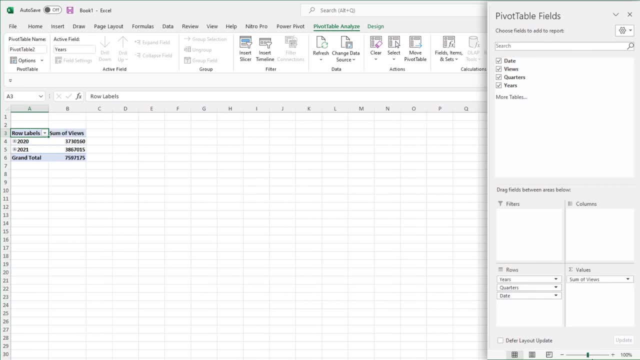 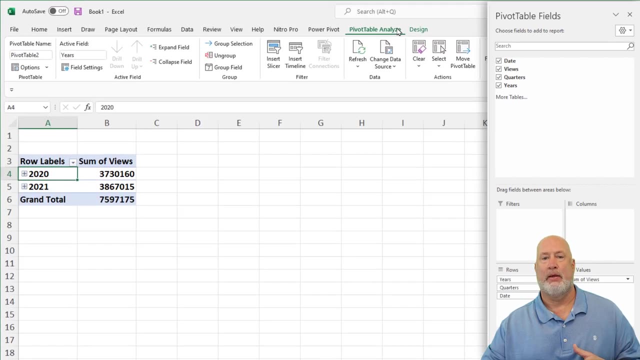 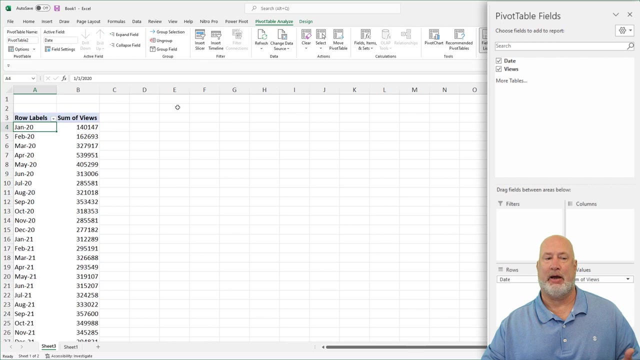 I'm going to check date. I'm going to check views. There we go, Zoomed in Just a tad Click on one of the dates. So I clicked on A4, pivot table. analyze the group tab. do an ungroup. So there are my 24 months again, by the way. 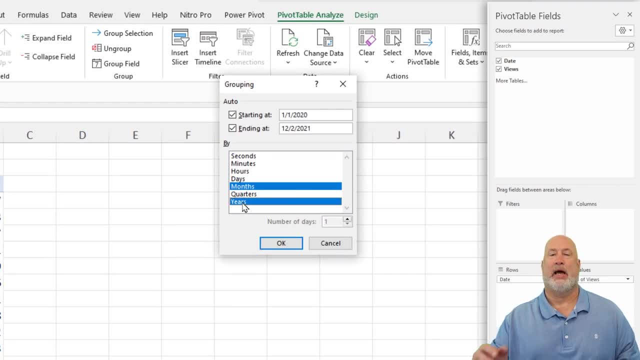 Now I go back to group. How do you want to group this? I could do quarters if I wanted to, because I just showed you Microsoft's quarterly year-to-year, but I want to do months. So I'm going to check months. I'm also going to check years, Click OK, There's. 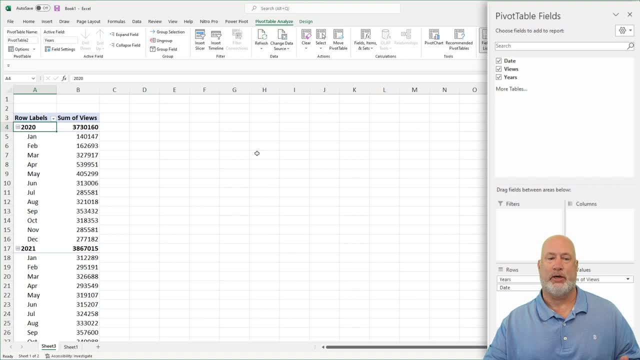 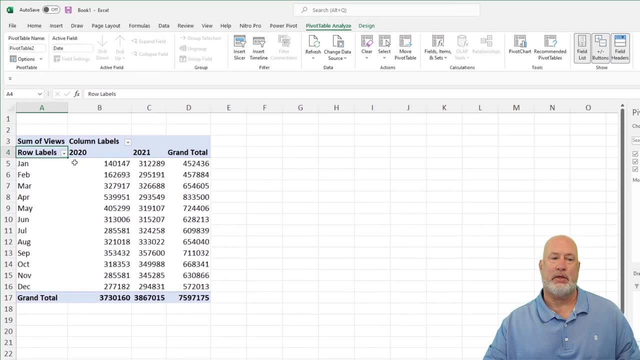 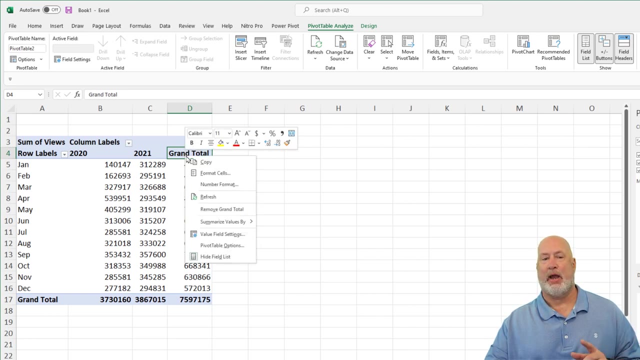 everything for 2020 and there's everything for 2021.. Drag years and drop it into the columns. All right, So there we go. The 12 months for two years grand total in column D is not needed. I'm going to right-click on cell D4 and remove it. 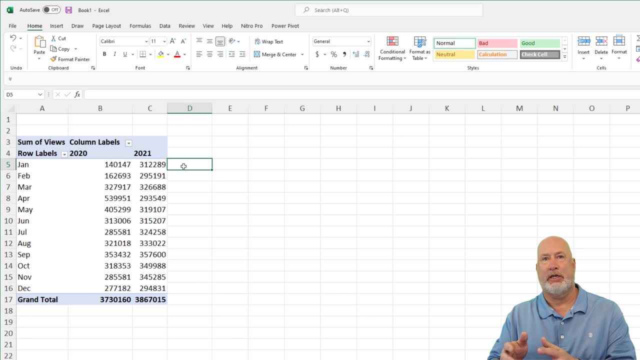 Now I could do the year-over-year percentage analysis right here by doing equals C5, device. right here by doing equals C5 divided by B5 minus one, that is 122% growth. But I want to do it inside the pivot table in case my data changes or I rearrange it. So this is the cool part of 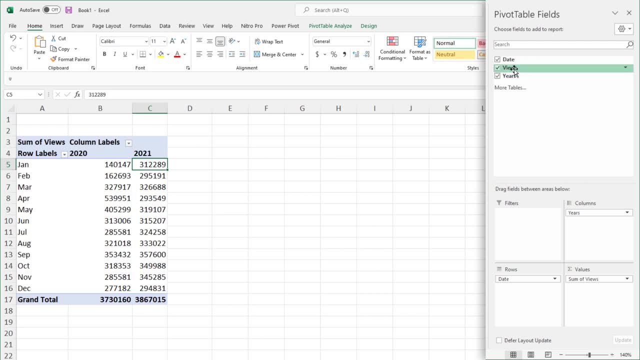 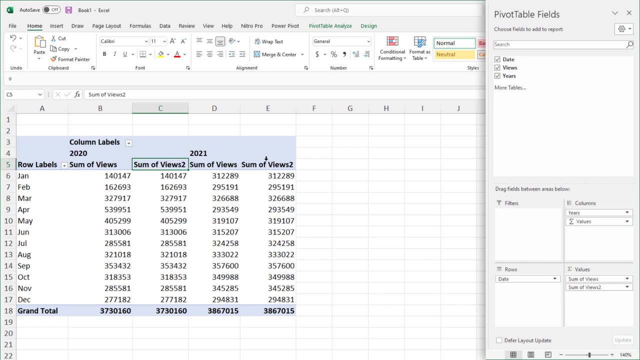 this video. I'm going to take Views again and again. it's whatever you want to look at. I'm going to drop it into the values again. So now I end up with at least four columns and I do next to the months one, two, three, four. That last column in E it says Sum of Views To: 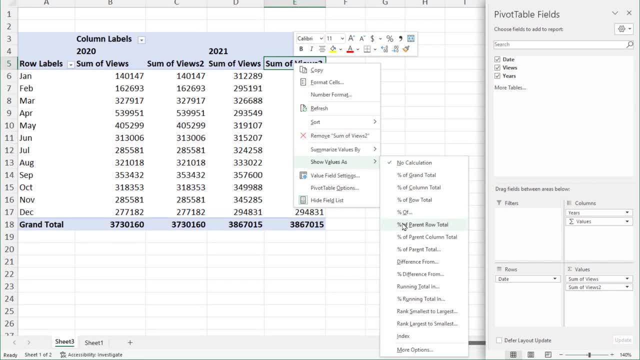 Right-click it, Show Value As and notice I'm going to go to Percentage Difference From. If I want to know the dollar difference, I would have done the one above it, just Difference From, but I want to know the percentage. 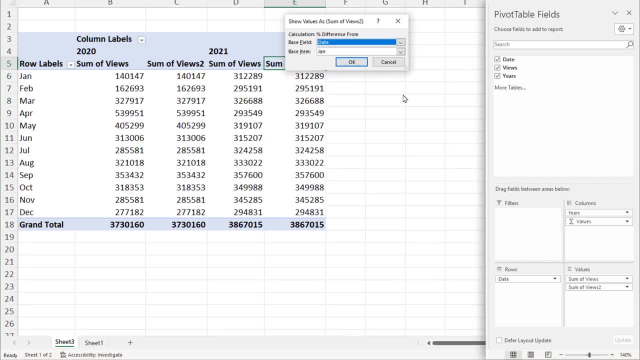 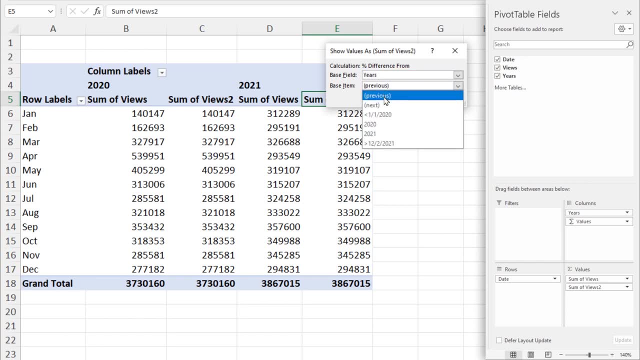 If you're recall, I got 122% a second ago. You want to make sure that this is years, not date, And base item is the previous year. So now when I hit OK in cell E6, I should see 122%, and I do. 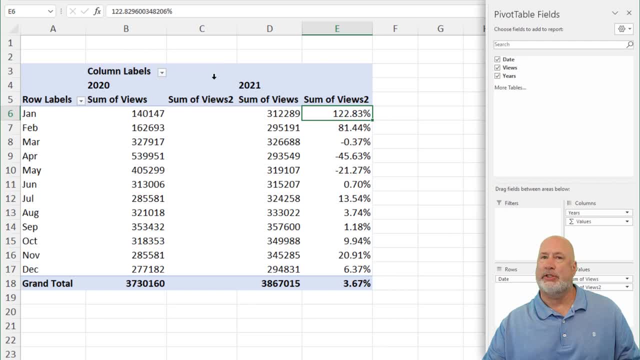 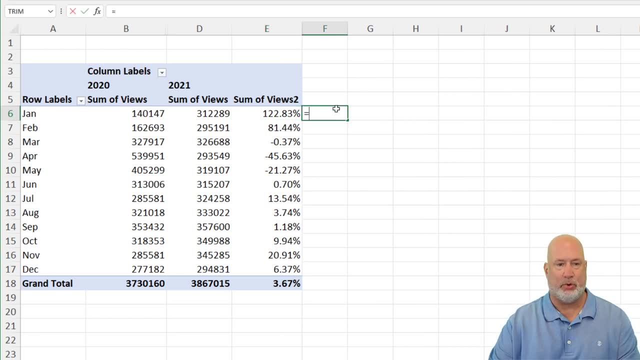 The key to this also is not only just doing what I just did, but column C you don't need. So here's the easy tip: just hide it. So there you go. I'm going to test these real quick. I'm going to go- exactly what I just did a second ago.